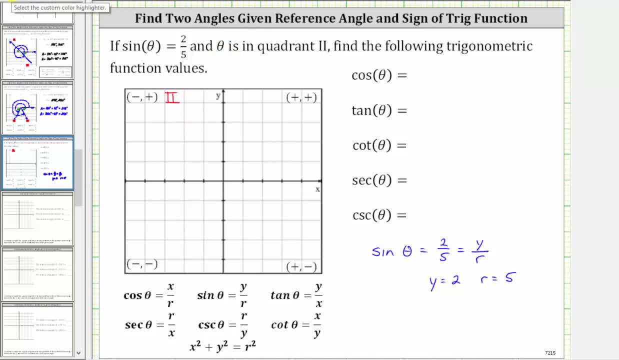 for angle theta in the second quadrant. Let's go ahead and assume this is the terminal side of our angle theta And therefore the reference angle is this angle here, formed by the negative x-axis in the terminal side. So let's call this theta reference. 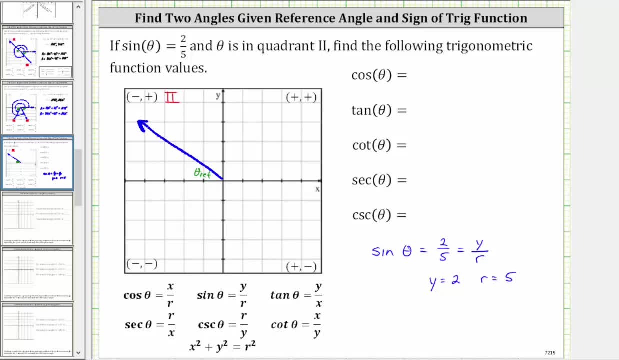 Let's also sketch the reference triangle. So let's go ahead and let this be the reference triangle. And because sine theta is equal to two fifths, we know the opposite side, or y is equal to two and the hypotenuse, or r is equal to five. 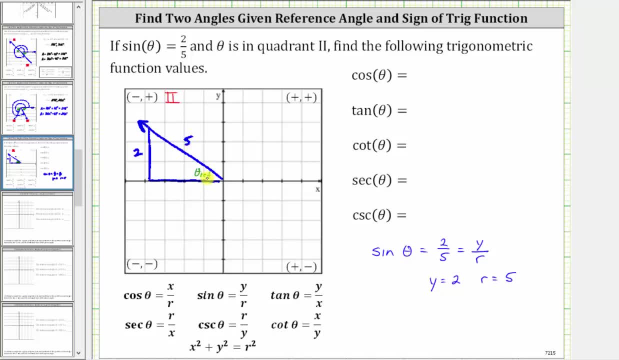 In order to find all the trigonometric function values, we will also need to determine x, which notice how, because we are in the second quadrant, we'll be negative. To determine the value of x, we will use the Pythagorean theorem. 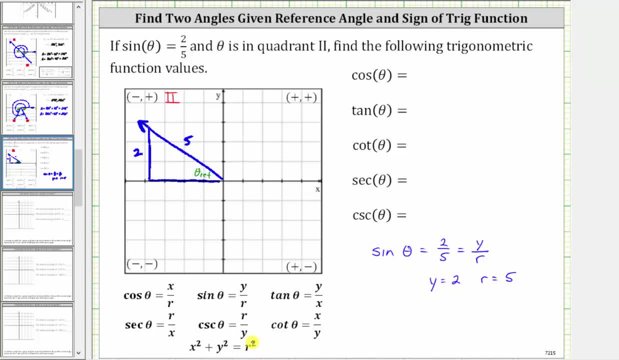 which is also the equation x squared plus y squared equals r squared. So, using x squared plus y squared equals r squared, we substitute two for y and five for r, which gives us x squared plus the square of two equals the square of five. 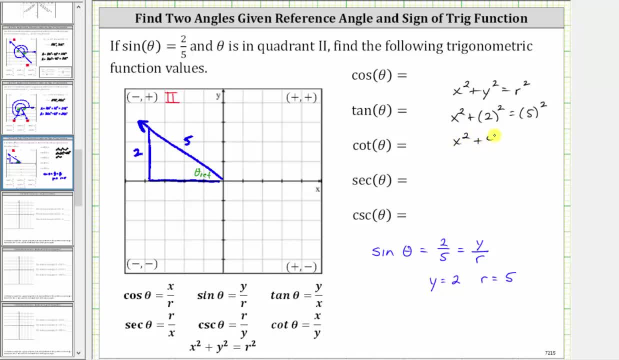 Simplifying, we have: x squared plus four equals 25.. Isolating x squared, we subtract four on both sides, which gives us x squared equals 21.. And now we take the square root of both sides of the equation. and when we do this, 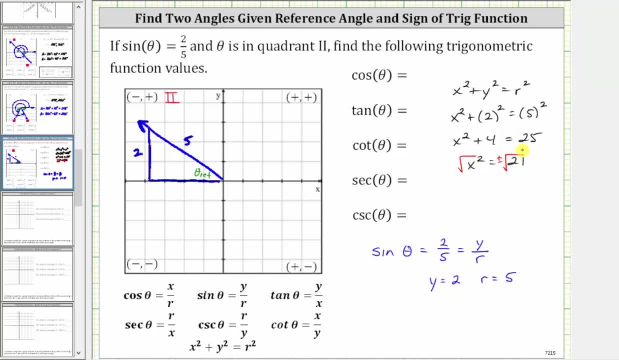 we include a plus or minus on the right, which gives us x equals plus or minus the square root of 21.. But we know x is negative because we are in the second quadrant and therefore we now know x is equal to negative square root of 21.. 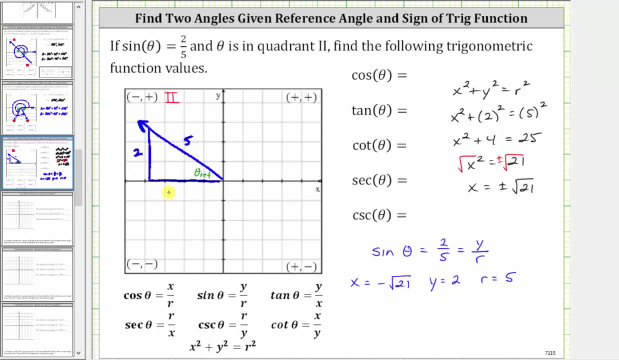 Let's also label this on the reference triangle, And now we have all the information we need. in order to find these five trig function values, We can either use the definitions of the trig functions in terms of x, y and r, or we can use the reference triangle. 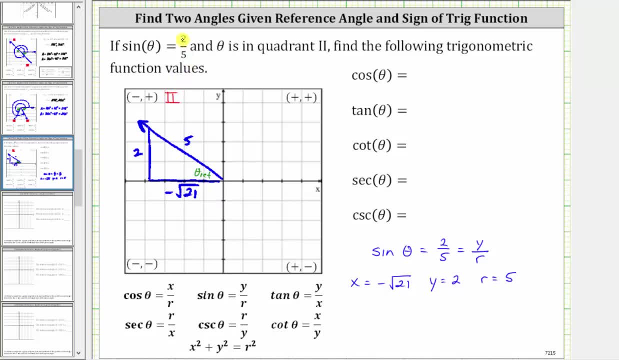 We will discuss both, To begin, because we know sine theta is equal to 2 5ths, and sine and cosecant are reciprocals of one another and therefore cosecant theta is equal to the reciprocal of 2 5ths, which is 5 halves.